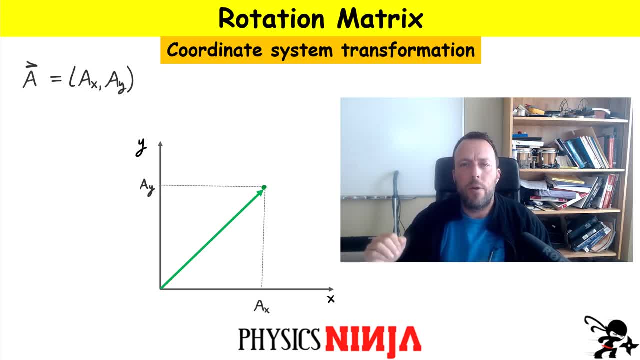 coordinate system. for imagine if you're designing a video game where there are multiple coordinate systems, maybe a global one and a lot of local coordinate systems. They might not be parallel to each other, Some may be rotated relative to each other. So imagine we have this vector here. 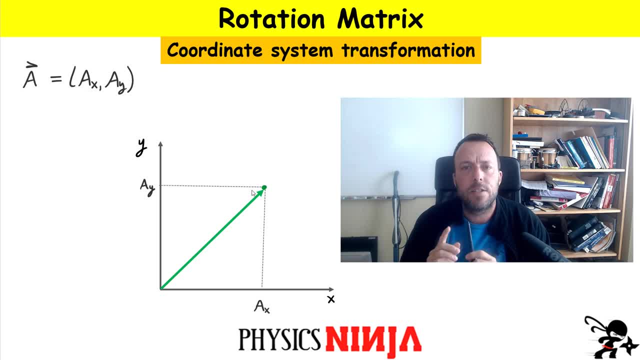 this green vector. It has a certain magnitude and it has components ax and ay in the global coordinate system. And what if I have another coordinate system and I want to rotate it, for example? right, It might look something like this: So I have a prime coordinate system drawn. 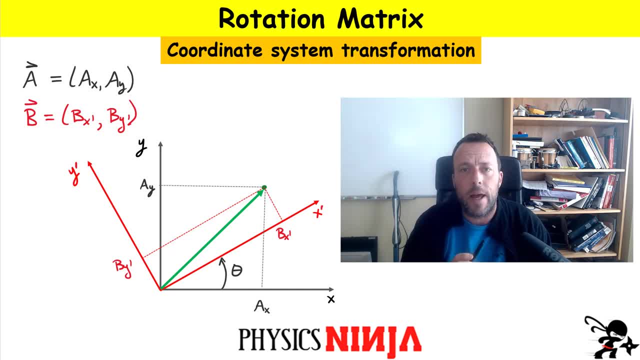 in red right. So I'm showing you the same vector. now It has components bx, prime and by prime in a different coordinate system. So what I want to do today is I want to look at how do I transform my coordinates ax and ay into the new coordinate system that is. 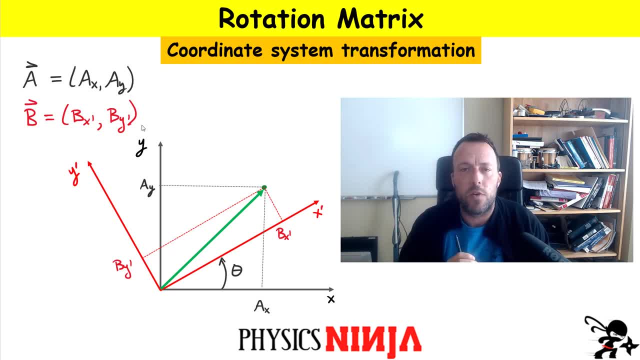 rotated by some angle theta relative to the first one. All right, we're going to go through kind of the simple proof of this. Now notice, I'm not rotating the vector. The vector hasn't changed or the point in space hasn't changed. I'm only rotating the coordinate system. in this case. 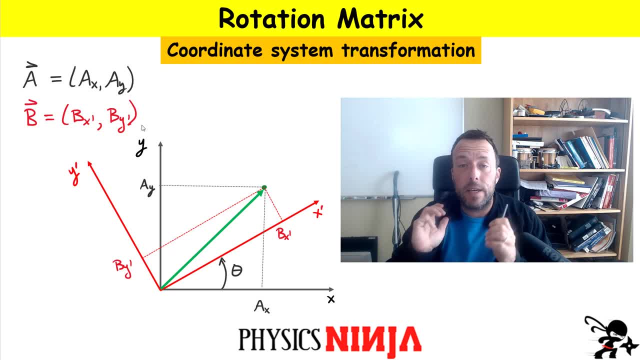 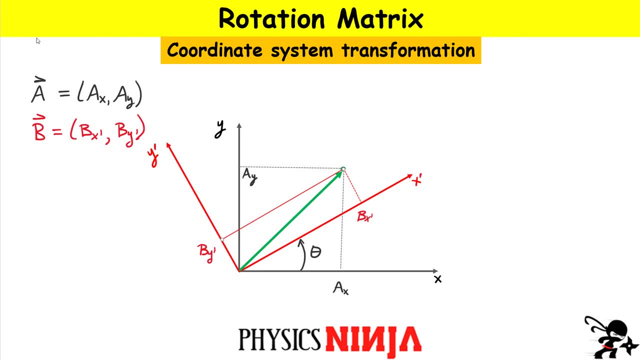 So it'd be a little bit complicated to do that, But I'm going to go ahead and do that, So be careful, Like with all my videos. if you like it, give it a thumbs up, Consider subscribing to my channel. Okay, let's get started. Okay, so here's the setup. We have our global coordinate. 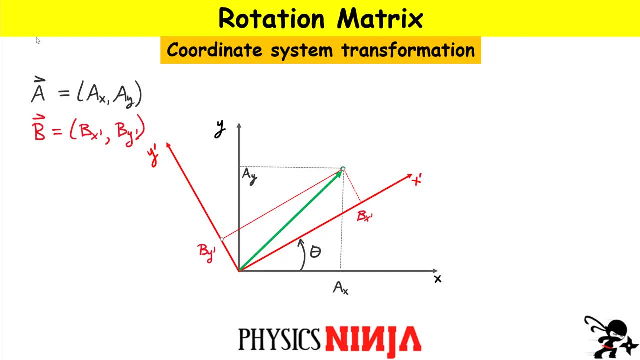 system with its two components and we have our rotated coordinate system in red with its two components. Now I'm going to show you at least. the easiest way to prove this, in my opinion, is to do it like this. So we notice we have our components here in red, We have bx. 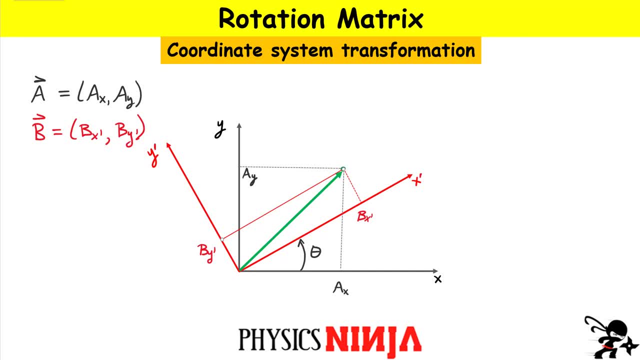 prime and by prime In order to prove this. I think the best way to do it is to do it this way: First, we're going to move one line over. I just want to add some extra lines because we're going to have to link all of these components together, And I just want to make the diagram as clear as 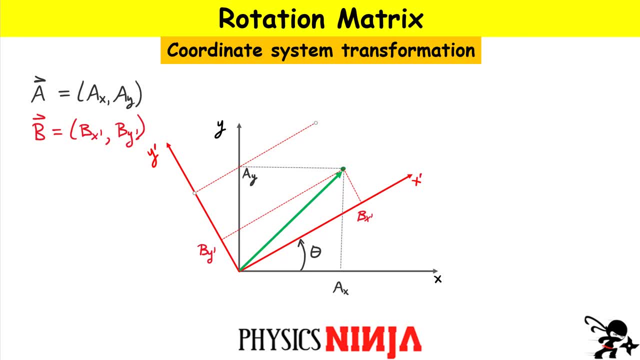 possible. So I make that line and I move it over and the total length of this line has to be bx prime, right, It's the same as over here. Now, the other thing I want to do now is just extend this line a little bit, okay, And the total length of that line we're going to be able to find, because 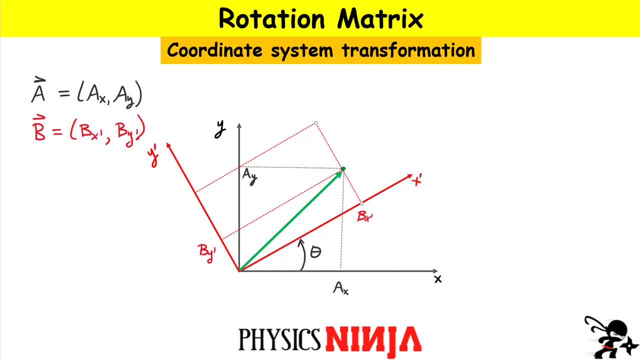 it's going to be the total length of the line here on the left hand side. Now I want to do that by notice a couple things about this diagram. There are a lot of triangles here, so let's just keep in mind a couple things. The value ax is this one right here. This is ax, right, It's the same as. 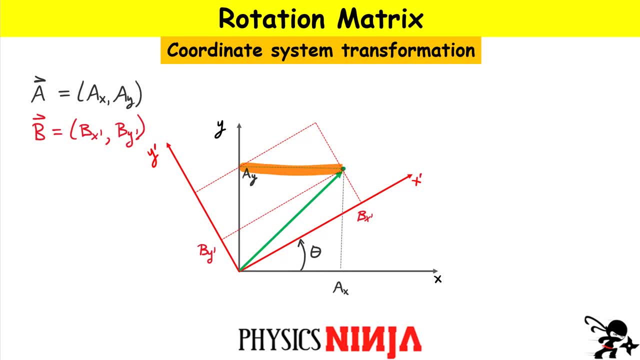 down here. okay, That has to be ax, Let's get rid of that. And the ay length has to be this one Ay. is this length right here, right, Measured on the global coordinate system y-axis? So keep that in mind. Now we're going to define some distances here. Now again, if this is the 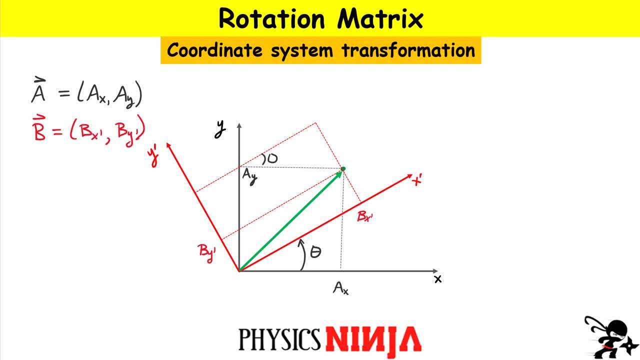 angle theta. you should be able to convince yourself that this here is also the angle theta. All right, now we're going to define some terms right here. First term we're going to define is: again, I'm going to also write the angle theta down over here. All right, so let's go ahead and 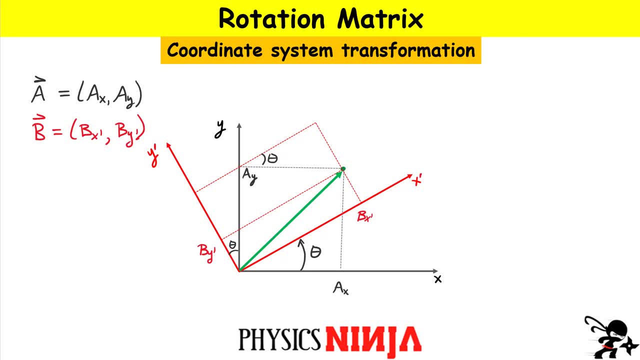 do some things. So we have: ax is the hypotenuse distance. That means that this distance right here, this here, must be ax cos of the angle theta. This side right here would then mean that this here is ax sine of the angle theta. Okay, we have a few more to do. 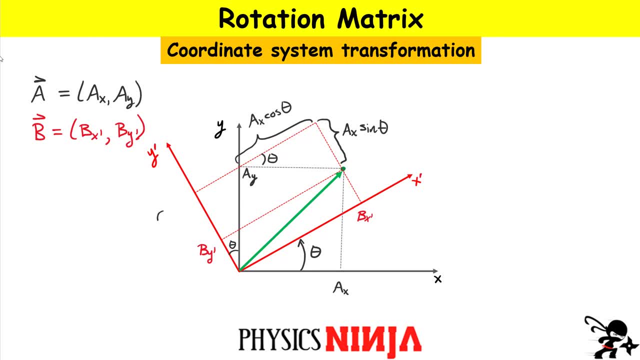 Let's go on this side. Remember: this whole length is ay. That means that this total length must be ay cos of the angle theta, which would mean that this little bit right here must be ay sin of the angle theta. All right, so if you can get to this point, you've pretty much done the. 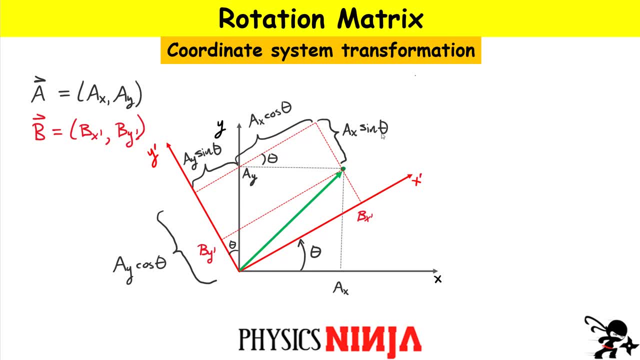 problem, Okay, Okay, so now we can start writing things out. So we're going to write down our x component, bx, prime, bx, prime. is this total length right here, which I've repeated at the top of that rectangle, right? That is the total length And you can see. now you can write it in terms of the. 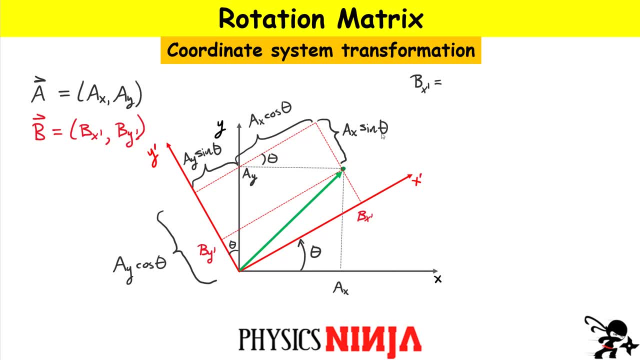 a components. So bx prime you should be able to write as ay sine of the angle theta plus ax cos of the angle theta. All right, what about by prime? By prime is a little bit more difficult. By prime is small right here, right, It's only this one. But again, you should be able. 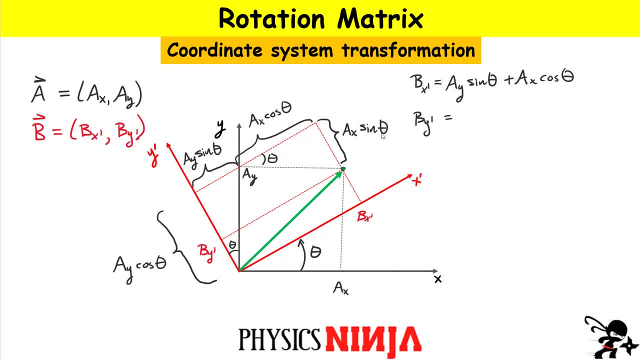 to write it as the total distance here minus this other section over here. So make sure you understand this. So this is ay cos of the angle theta and then minus ax sine of the angle theta. All right, so what we're going to do now is simply just rearrange terms and then we'll write it in. 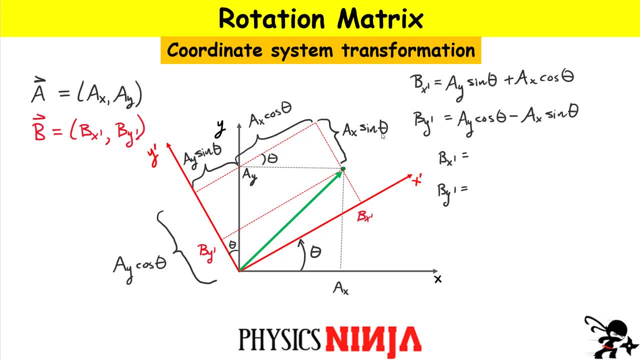 matrix form To rearrange terms. I'm just going to put the x components first. So we're going to have cos of the angle theta multiplied by ax- I just swapped the order here- Plus sine of the angle theta multiplied by ay. And for the prime term, again I'm going to put the x component first. I. 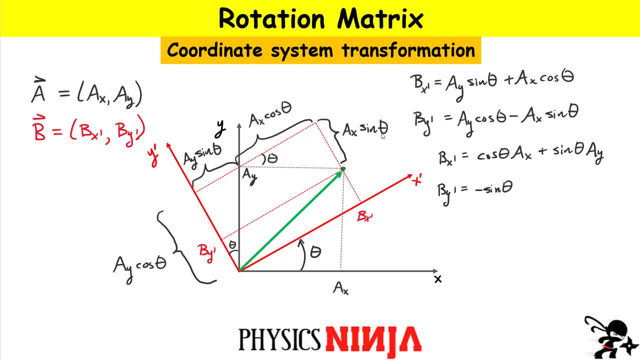 have a negative sine for the sine theta, term ax And then plus cos of the angle theta multiplied by ay. Now you can see right away. you can write this in matrix and vector form. All right, these are the components of my b vector, And then I can. 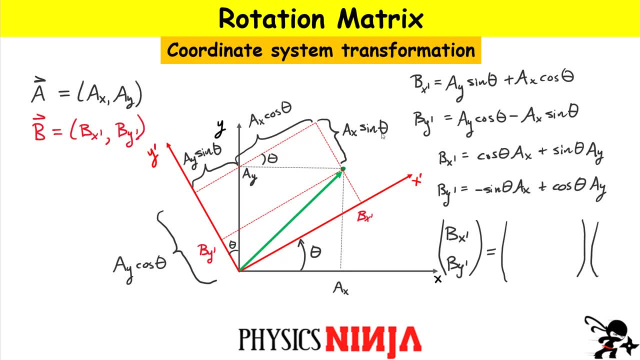 introduce a rotation matrix and that gets multiplied by the components of the global coordinate system, ax and ay. All right, if I have a look at the two equations I have here, you should be able to write this as cos of the angle theta. 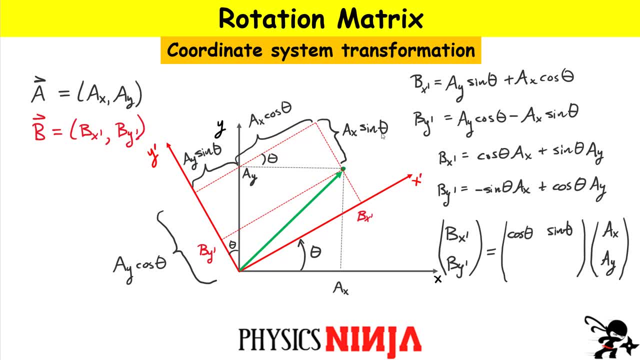 sine of the angle theta, minus sine, and then cos of the angle theta. Okay, so at the end you can write down that this vector could be equal to this rotation matrix multiplied by the vector a. Okay, and my rotation matrix for this problem is simply this guy. Okay, so that is how you can rotate one set of coordinates. 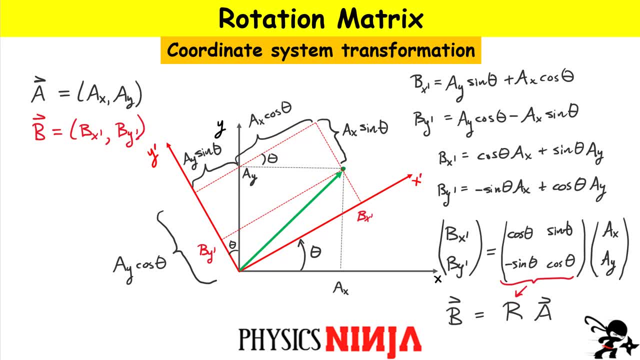 relative to another. Okay, so that is how you can rotate one set of coordinates relative to another. Okay, so that is how you can rotate one set of coordinates relative to another, Just using this simple proof. All right, one thing I always do after getting a result is check it using 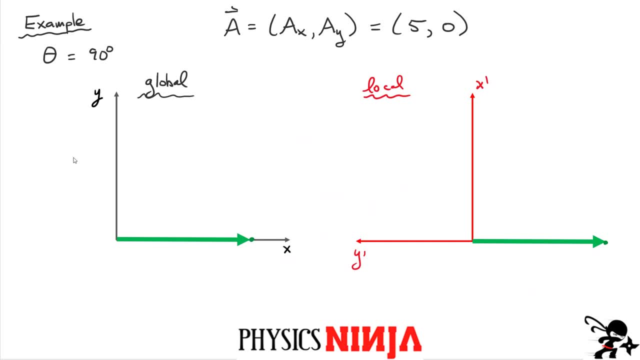 some very, very simple cases. So here we have our global coordinate system, And I'm going to take a very simple vector that simply lies along the x axis. here It has a magnitude of five. All right, what if I rotated now a coordinate system by an angle equal to 90 degrees? So again,